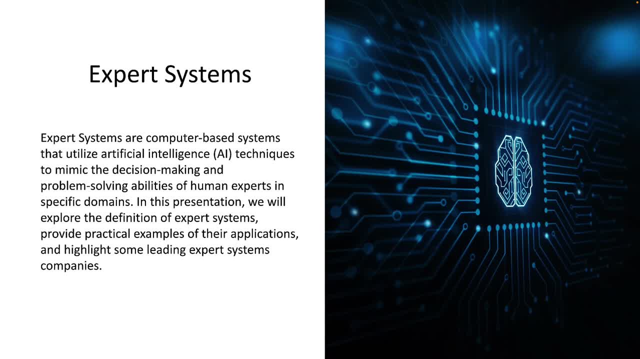 artificial intelligence or AI, techniques to mimic the decision making and problem solving abilities of human experts in specific domains. In this lesson, we're going to look at the definition of expert systems, look at some practical examples of their applications and highlight some of the leading expert systems companies. So let's go ahead and take a look. 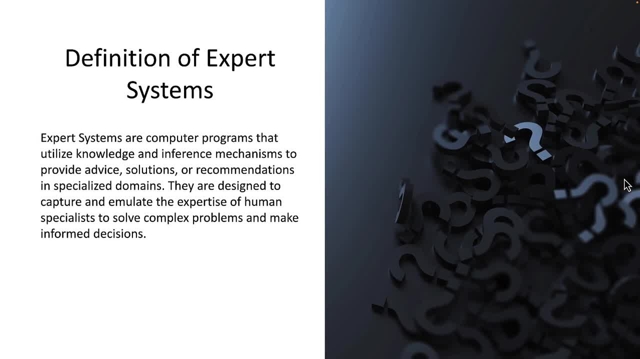 at the rest of the material. So let's start off with a definition of expert systems. Expert systems are computer programs that utilize knowledge and inference mechanisms to provide advice, solutions or recommendations. Expert systems require a technician to cover a specific issue or program. and là d'NOISE. 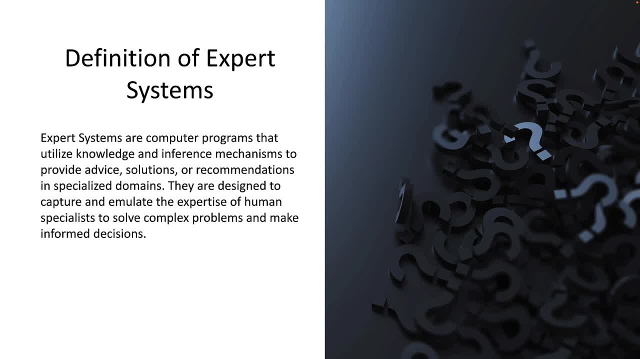 d'Air. Expert systems are computer programs designed by experts in their respective domains. They'll influence and limit solutions and solutions throughout a particular domain. ić Expert systems are science based processing and estimating too, Ram mentioned in this last point, but they're a form of error verification. 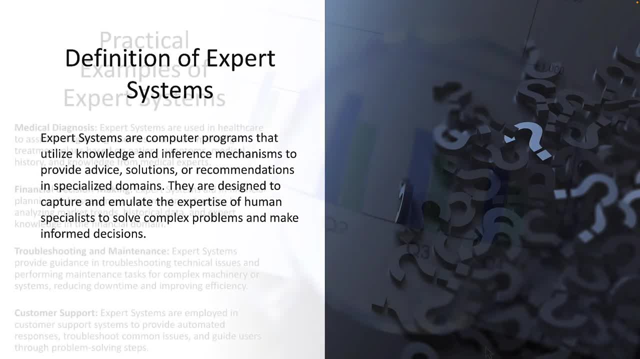 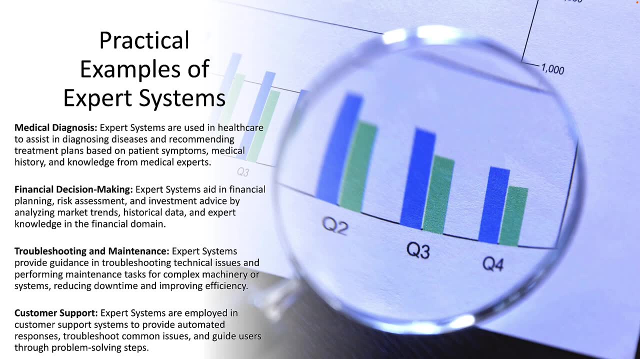 Expert systems may be designed to capture and emulate the expertise of a human specialist to solve complex problems and make informed decisions. look at some practical examples of expert systems. The first one: we talked about medical diagnosis. Expert systems are used in health care to assist in diagnosing diseases and recommending treatment. 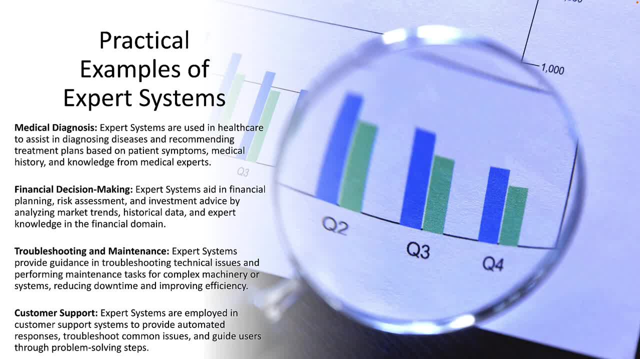 plans based on patient symptoms, medical history and knowledge from medical experts. The next one is financial decision making: Expert systems, aid in financial planning, risk assessment and advice. investment advice by analyzing market trends, historical data and expert knowledge in the 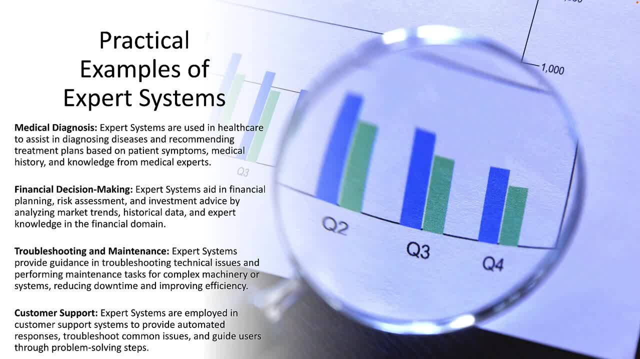 financial domain. The next one is troubleshooting and maintenance. Expert systems provide guidance in troubleshooting technical issues and performing maintenance tasks for complex machinery or systems, reducing downtime and improving efficiency. The last one is customer support. Expert systems are employed in the customer support systems to provide automated responses, troubleshooting. 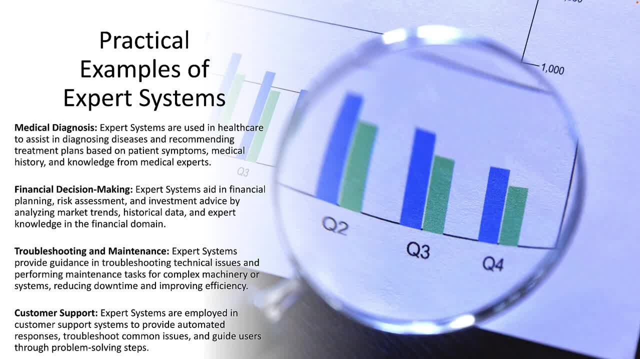 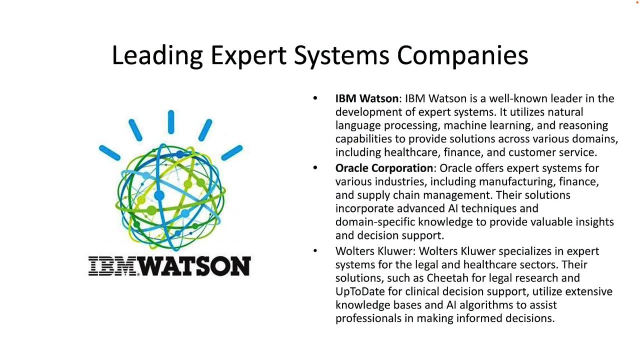 common issues and guiding users through problem solving steps. So there's four very practical examples of expert systems. Let's look at some of the leading expert system companies that are in the market today. The first is IBM Watson. IBM Watson is a well-known leader in the development of expert systems. 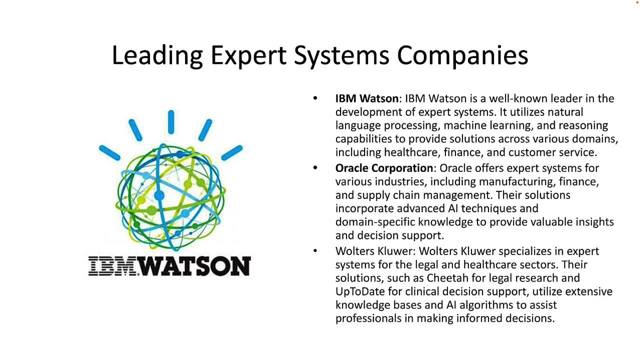 It utilizes natural language, processing, machine learning and reasoning capabilities to provide solutions across various domains, including health care, finance and customer service. The next one is Oracle Corporation. Oracle offers expert systems for various industries, including manufacturing, finance and supply chain management. Their 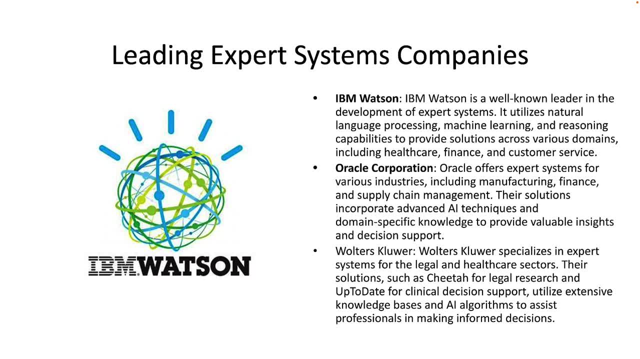 solutions incorporate advanced AI techniques and domain-specific knowledge to provide valuable insights and decision support. The last one is Walters Kluwer, And Walters Kluwer specializes in expert systems for the legal and healthcare sectors. Their solutions, such as Cheetah for 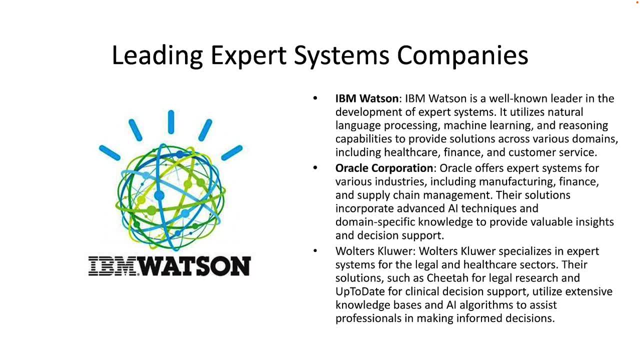 legal research and UpToDate for clinical decision support. utilize extensive knowledge bases and AI algorithms to assist customers in their decision making and decision making processes. The last one is Intel. They have developed a complex distribution of AI technologies such as approximation math and Mechanical Math. The larger version is called the Intel i7. Intel's 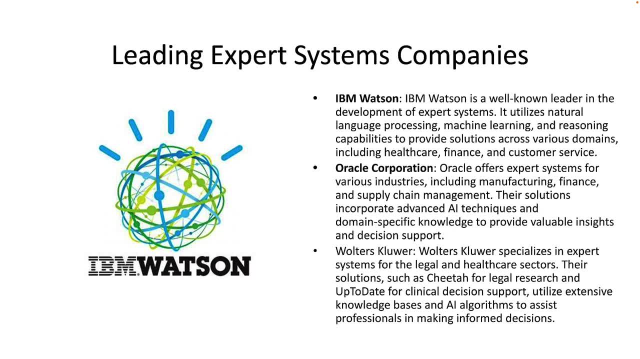 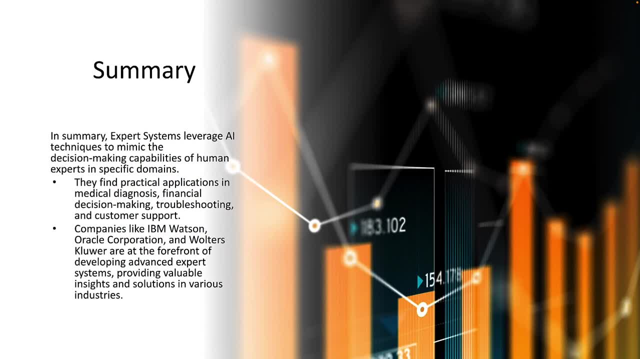 systems are more complex than the Apple i7, and the Intel i7 is more complex than the Apple i6.. When it comes to making decisions, they require a wide range of skills. The added purity and complexity of AI is a great example of the high quality of AI. 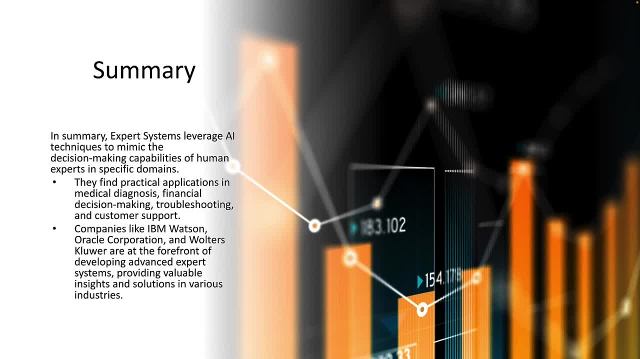 But there are only a few examples in the market today that are considered to be the best in terms of quality: The advanced AI technology professional development system. consultations are particularly powerful in the field of AI analysis professionals and making informed decisions. I should note this is. 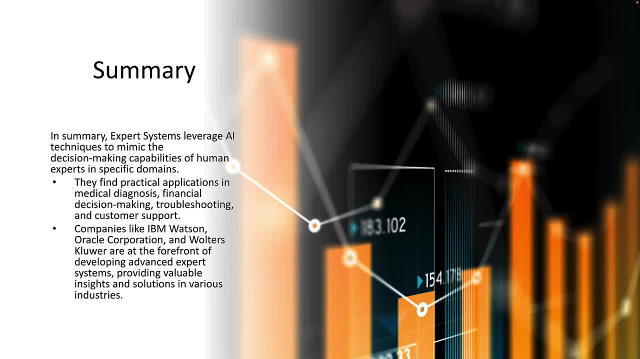 just a small sample of the literal flood of products that are out there based on AI and expert systems, But these are three pretty well-known examples of some of the leading companies in this space: decision-making, troubleshooting and customer support Companies like IBM Watson, Oracle. 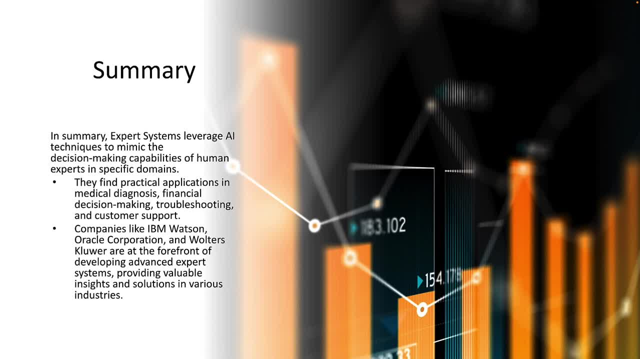 Corporation and Walters Kluwer are at the forefront of developing expert systems and providing valuable insights and solutions in various industries. Well, that's it for this lesson, with our brief look at expert systems. That's all for this lesson. Thank you so much. 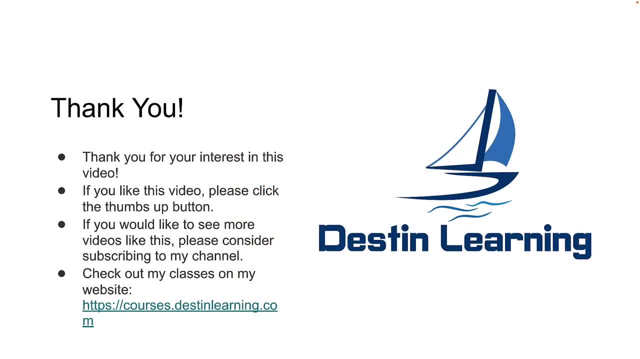 and I'll see you in the next lesson. Bye-bye. Thank you for your interest in this video. If you like this video, please click the thumbs up button. If you'd like to see more videos like this, please consider subscribing to my channel, and you can check out my classes on my website. 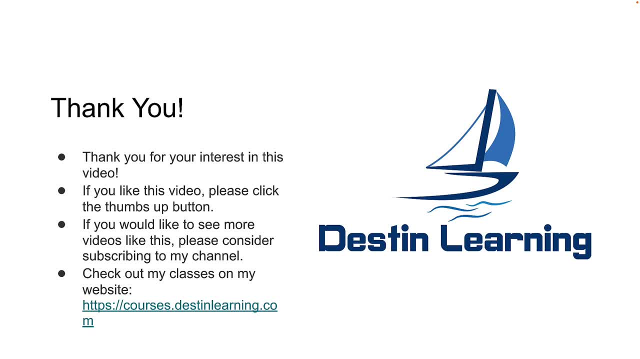 at coursesdestinlearningcom. Thanks again and I'll see you again soon. Bye-bye.